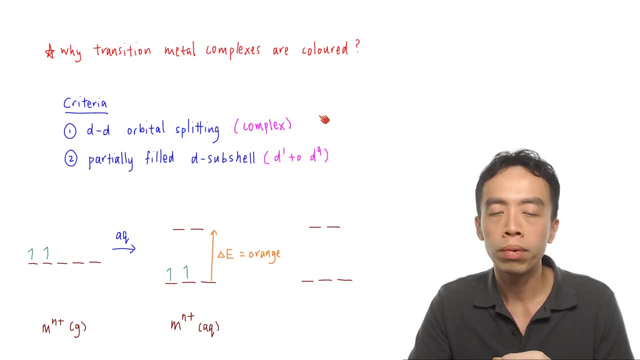 So the dd, orbital splitting, usually is linked to complex formation. Now the second criteria is: I need to have a partially filled d subshell. I know that d subshells can hold up to a maximum of 10 electrons. If there are no electrons, then the transition metal will not be colored. 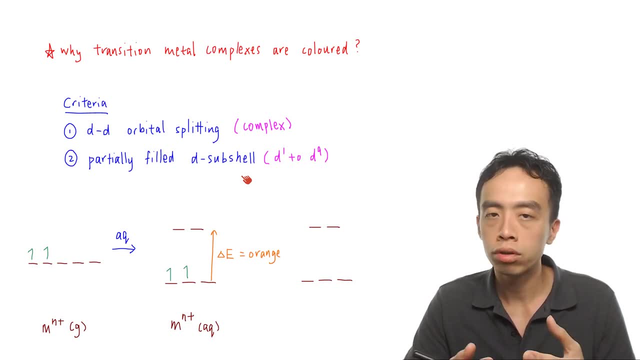 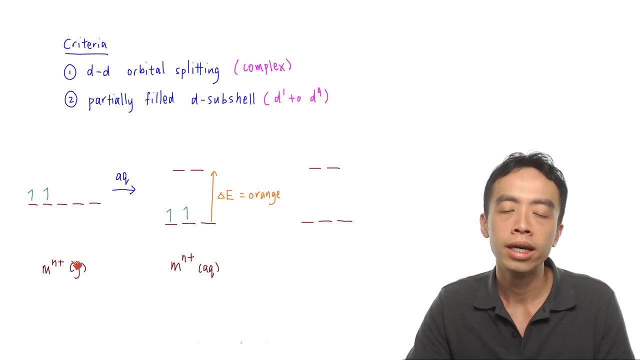 If it is fully filled d10, the transition metal will also not be colored. So partially filled d subshell would mean that the number of electrons in the d subshell must be between d1 to d9.. Alright, next let's look at an example involving Mn plus in the gaseous state And let's say for: 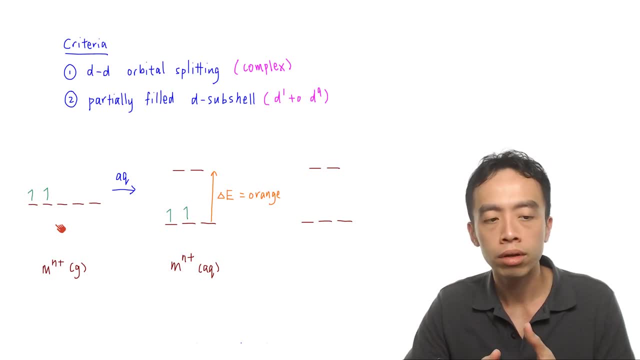 example, it has two electrons in the d subshell. Now you notice, when it has two electrons in the d subshell, it actually fulfills the second criteria. I have a partially filled d subshell because it is d2 between d1 to d9. But it doesn't have any. 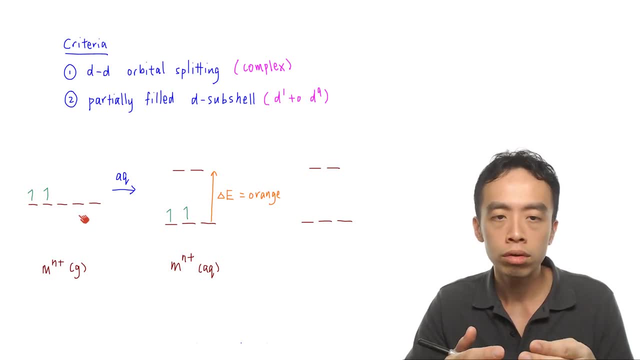 dd orbital splitting. So there's no difference in energy level. So therefore there's no transition involved. And Mn plus in the gaseous state it is colorless or it doesn't have a color. So what happens if I throw this Mn plus gas into solution and it forms a complex with water? 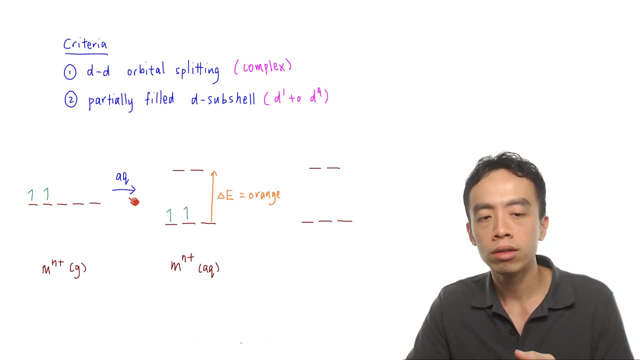 Usually we will form an octahedral complex and the splitting pattern will be two orbitals on top and three orbitals at the bottom. So you notice we have this energy gap, delta E. In terms of arranging the electrons, by default we will put the electrons in a lower energy state. 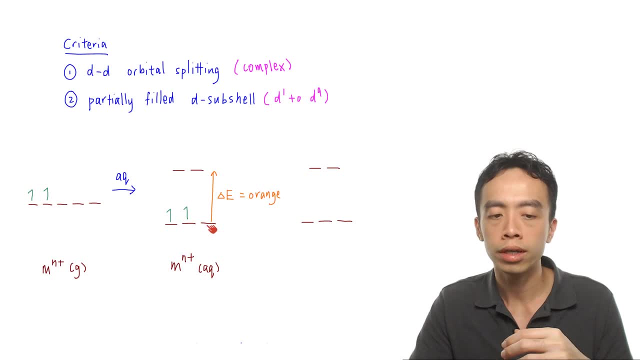 So these two electrons will be at the bottom, two electrons here. Then you notice now both criterias for transition metal complexes to be colored will be there. The first thing is I have a dd orbital splitting which will be here. I have a lower energy d level and a higher energy d level. 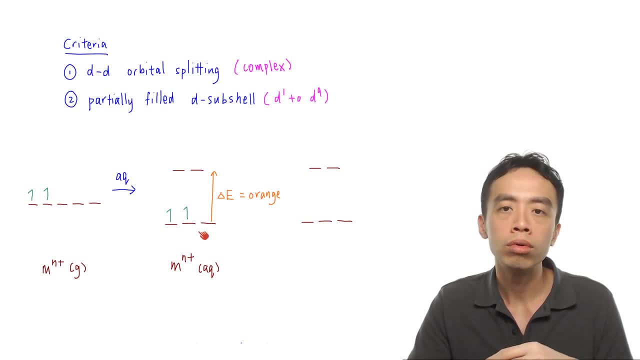 And the second thing is I have a partially filled d subshell, two electrons in the d subshell. Now what happens? This energy gap actually corresponds to a particular color that we can observe, which is in the visible light region. So, for example, let's say the color which corresponds. 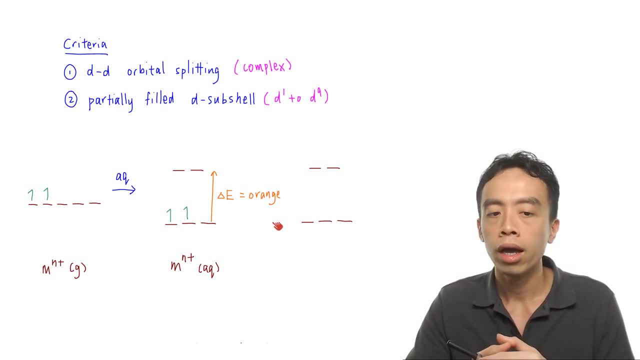 to this energy gap will be orange color And what the electron at the bottom can do is this electron at the bottom. it can actually absorb this orange light or the energy level that corresponds to this orange light, and it gets promoted. It can jump from the lower energy. 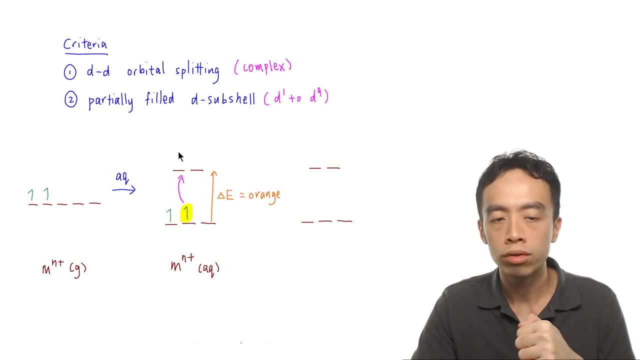 state to the lower energy state And then it can actually absorb the energy level that corresponds to this orange light. So once it gets promoted and jumps to this level, here ends up with something like this: I'll have one electron which stays at the bottom, And this electron, which is originally 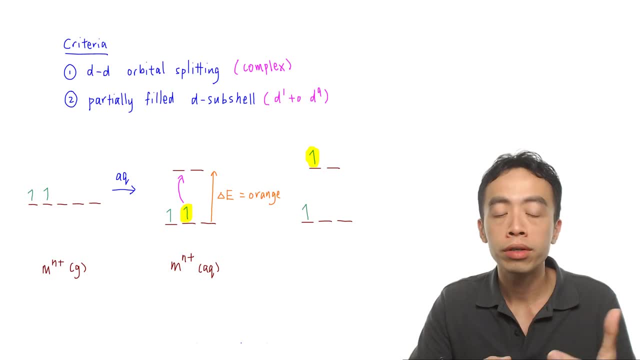 at the bottom. here it gets promoted on top. Now, what it has to do to change from this configuration to this configuration is it has to absorb orange light and it gets promoted from the lower energy state to a higher energy state. And because this orange color it is being 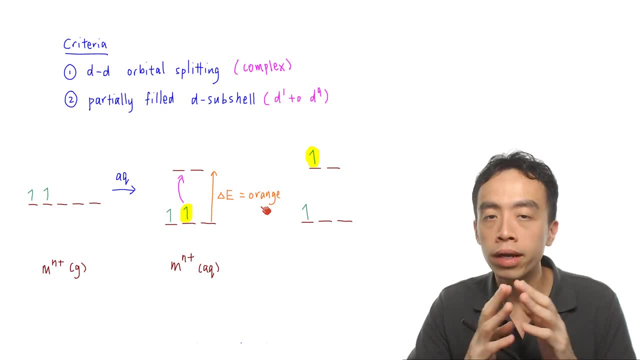 absorbed by this electron. so if i see this complex, i will not be able to detect the orange color because it is already absorbed, so i'll just see the rest of the colors. so in very simple terms, this explains the color of transition metal. so when we shine white light into this complex, 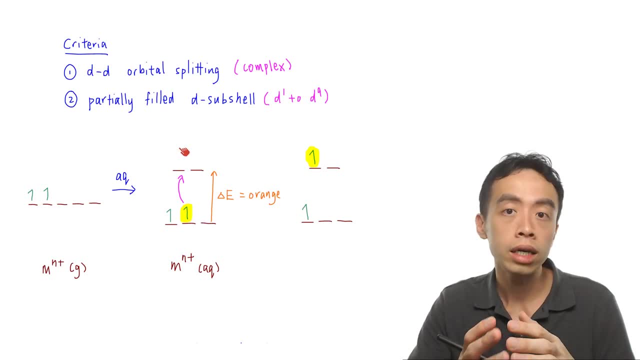 the electrons will absorb orange light and gets promoted to a higher energy state. so orange light is being absorbed away and the rest of the colors will be detected by us. so we will see this complex as the rest of the colors that is not being absorbed. so essentially, 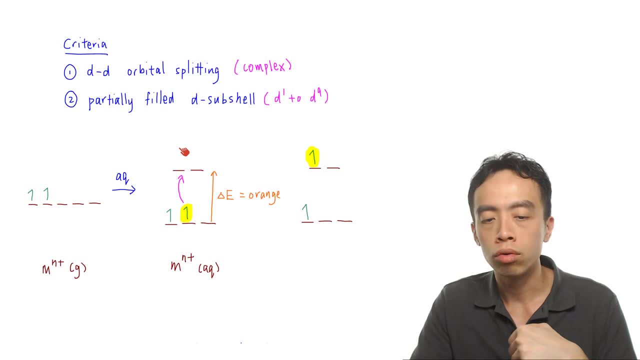 we will see the color which is complementary to this orange color. remember, if this complex absorbs orange light, i don't see the complex as orange light because the orange color is being absorbed away. so you see the rest of the colors. so it was essentially. we have this here in the 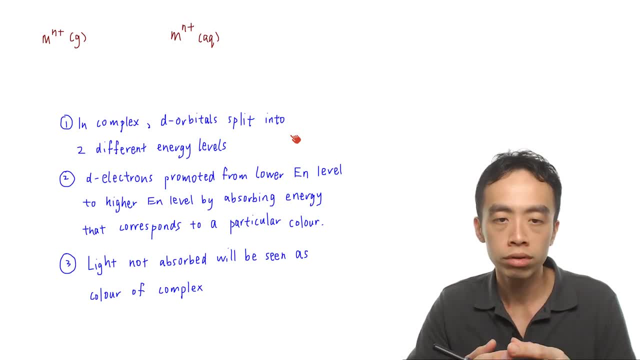 complex. the d orbitals will be split into two different energy levels: a lower energy level and a higher energy level. so the d electrons are promoted from a lower energy level to a higher energy level by absorbing energy that corresponds to a particular color. In the case of our example, you absorb orange light and it gets promoted from. 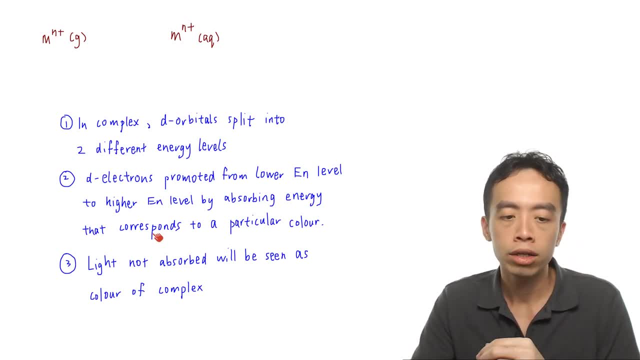 a lower energy state to a higher energy state, then light not absorbed will be seen as the color of the complex. That means if orange is being absorbed away, we will not be able to detect orange color. we will see the rest of the colors or the complementary color. Now we actually have 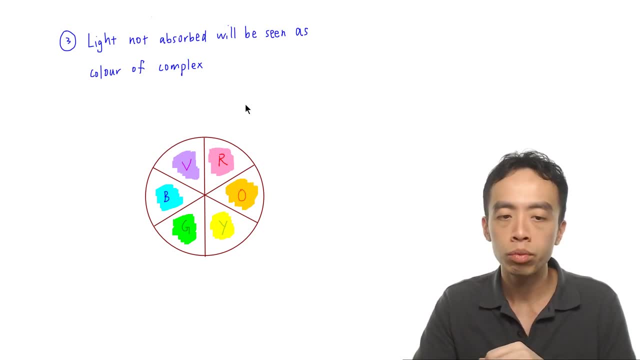 a way to predict the complementary color if I have this color wheel here and I cut it into six pieces and I just write down the colors of the rainbow- Actually, rainbow, usually we say that there are seven colors, but indigo and violet, they look somewhat similar. maybe we lump them together.